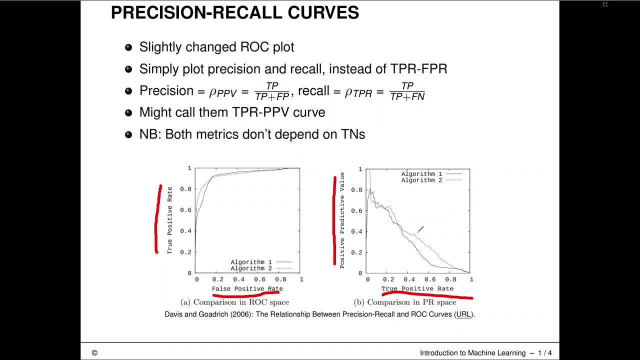 recall and the PPV the precision, And that's why that plot is called precision recall curve. Here I have given you the formulas for PPV and for TPR So we can maybe take a look at that. So if this is your confusion, matrix here and maybe here we have the y hat, Here we have the true y, Maybe we have the. 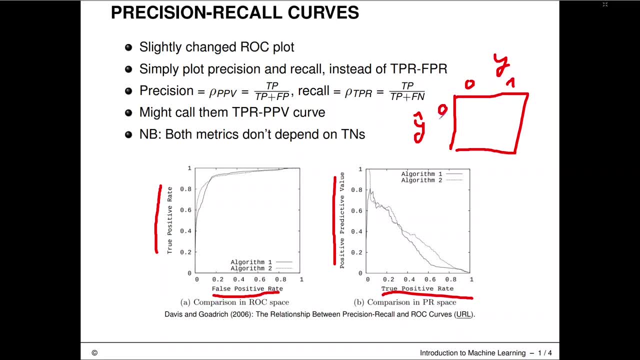 negative class here and the positive here. Here we have the predicted class, and here we have the predicted positive class. And then we have our two by two cells in our confusion matrix. Plot this guy here. What you're going to consider is a percentage in this column and in this column, And here we 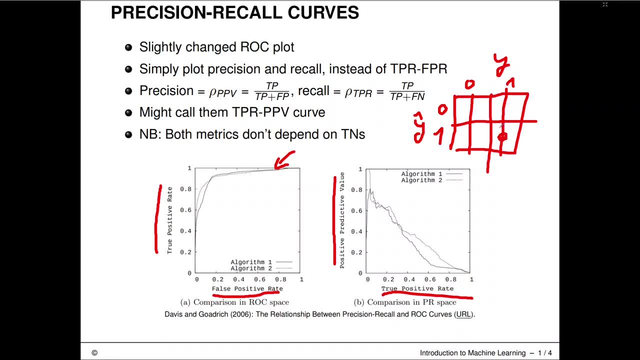 have now the true positive rate as a percentage in that column And we have the false positive rate- which is this guy here- as a percentage in this column. What we are doing in the precision recall curve is that again we consider the true positive rate as a percentage. 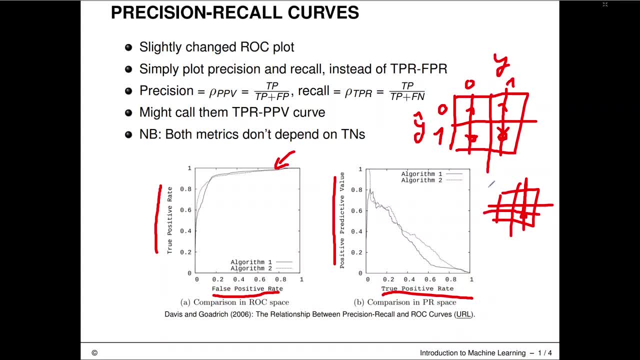 in this column. But we also consider positive predictive value, which is, given that we have predicted a one, It really is a one. So that's the percentage in this row here. Precision recall curve does not depend on this guy, So it doesn't depend on the true negative rate. But if you're plotting, 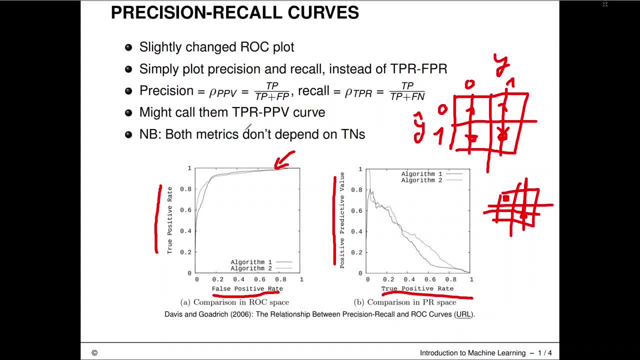 something in 2D. you have to make a choice which matrix you're going to use. You are plotting and there are usually three of interest. So the fourth one we can always compute. We could in principle compute from three given ones, But yeah, as usually these plots are, 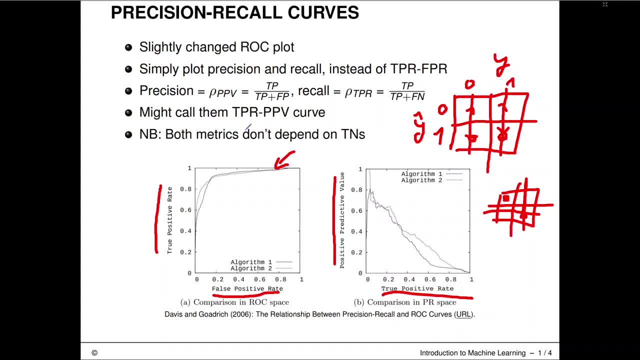 in 2D. you have to make a choice: which of the two you want to look at, And especially in highly imbalanced situations, as we'll figure out in a few seconds- precision recall curves might be the better choice. So this is exactly what I want to show here. So on the left hand side, 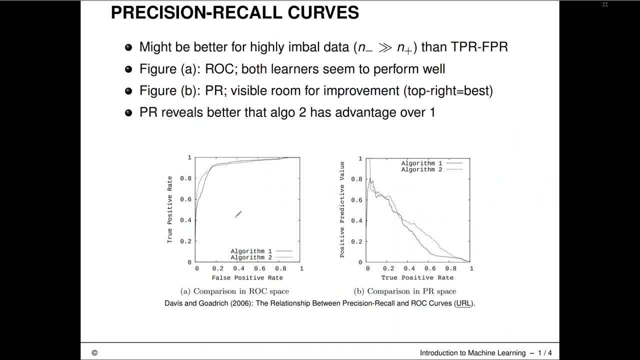 you have again. well it's. I guess we're going through that plot here multiple times, So we are going to study this a bit more in detail. So on the left hand side you see the standard ROC situation for two learning algorithms. now- And this is this- is quite imbalanced, So the negative class is quite a lot larger than the. 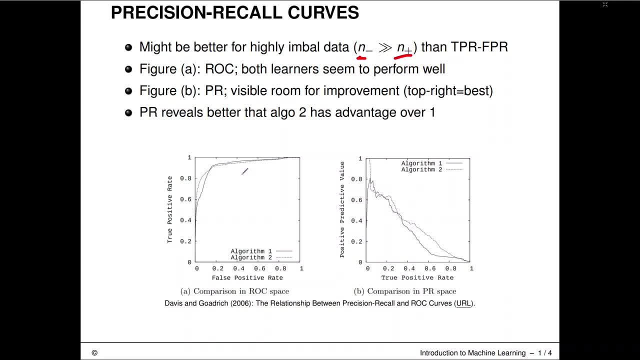 positive one. You could now conclude two things from this ROC plot for this situation here. that is that- And this is because both curves are somewhat close to this guy here, to the ideal point in the upper left corner, And both look also pretty much the same. So you can see that the 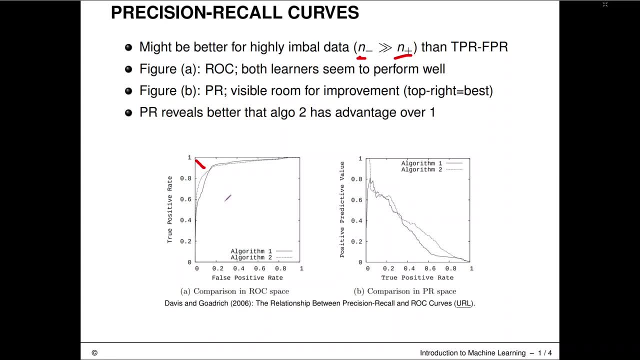 two are pretty similar. So we could conclude that both curves in both learning algorithms, both probabilistic binary classifiers are quite okayish And that there's also not a big difference between the two. Well, if you have a look here at the same situation now visualized through, 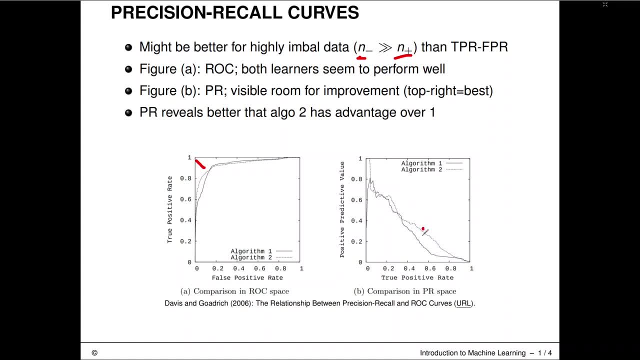 the PR curve, you can first of all see that there might actually be a bigger difference between the two guys, But what is maybe even more important is that both are actually far from ideal. So if you have a look here at the same situation now visualized through the PR curve, you can see. 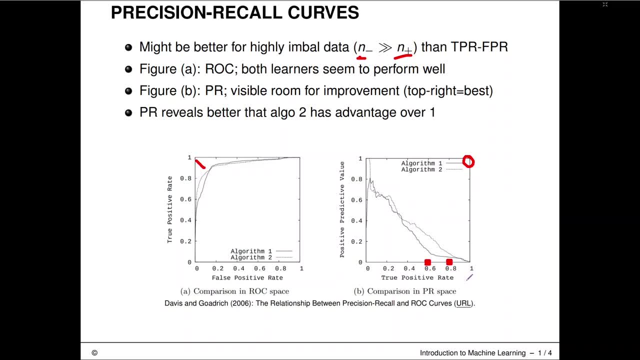 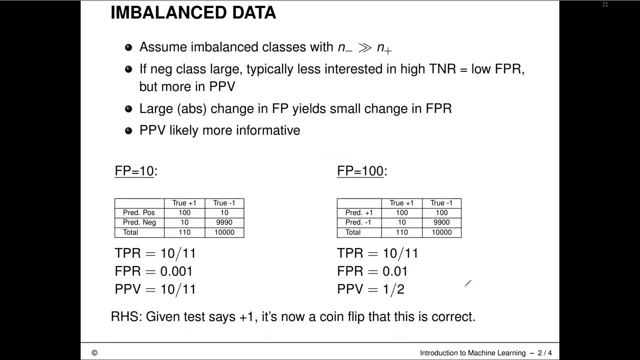 that both of these learning algorithms have now PPV scores which are even worse than a coin flip, So which are worse than 0.5. So they're actually not pretty good. Here's a further calculation for a similar situation. So again, a fairly imbalanced scenario If we take a look at the same situation. 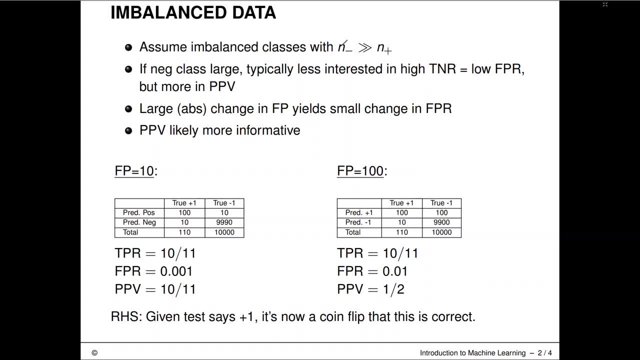 here we can see that both of these learning algorithms have now PPV scores which are even worse than a coin flip. So if we have a look here at these two confusion matrices, we can see that in both cases we have 110 cases in the positive class and 10k observations, So much larger set for the negative. 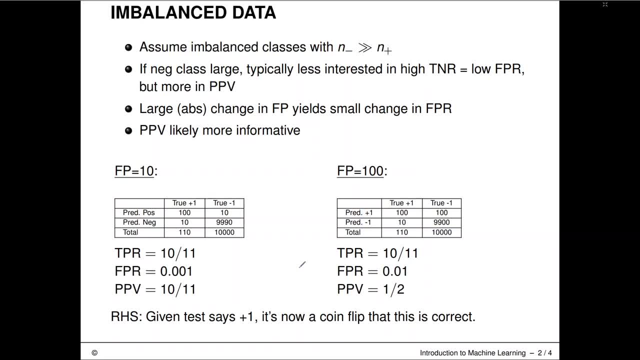 class, And both of these numbers are the same on the right hand side here, which is also the same in both situations, is the true positive rate. So that's roughly 90 percent. So we have about 90 elements, So 100 from 110.. 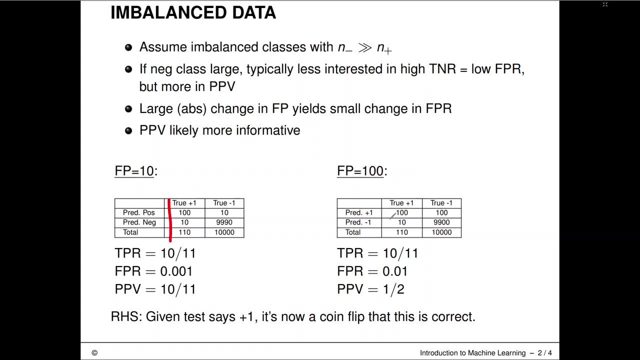 And 10 in this column here, And that's also not changed between these two situations. here We have 10 from 10,000. So an FPR of 0.001 of false positives And here the false positives are increased by a factor of 10.. But if you kind of look at the change in FPR, that could look to you. 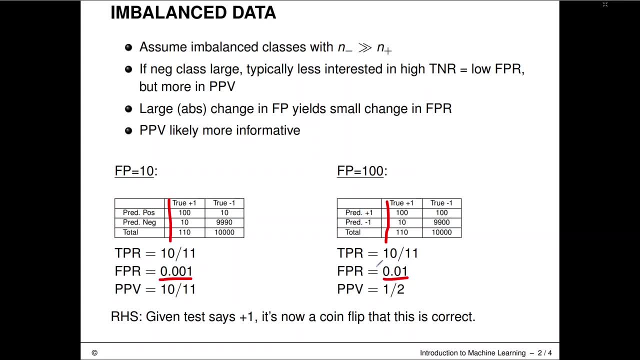 quite small, And this is the true positive rate in both cases we might deem as being good. Now the FPR also kind of looks good in both situations because it's a quite small value, close to zero, while on the left hand side we have a pretty nice positive predictive. 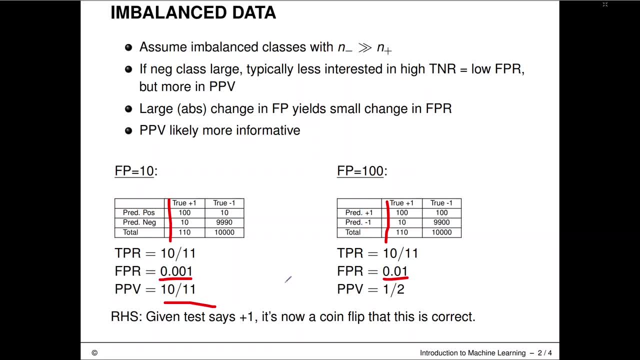 value. So if you would implement that test and assuming the test says yes, for example, you have the disease in the biomedical context, then here, with roughly 90 percent probability, you also truly have. You have the disease. So this is considering this row here. 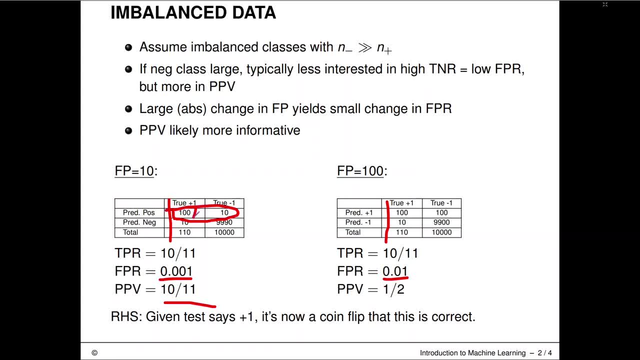 So we are predicting something to be positive. So we are in this cell and from 110 cases, 100 are correct. Now if we consider the same metric here on the right hand side, you can see it's 50: 50. So the PPV of our right hand side is as good as a coin flip. 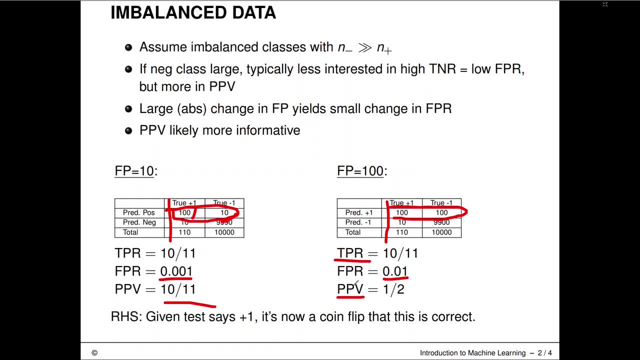 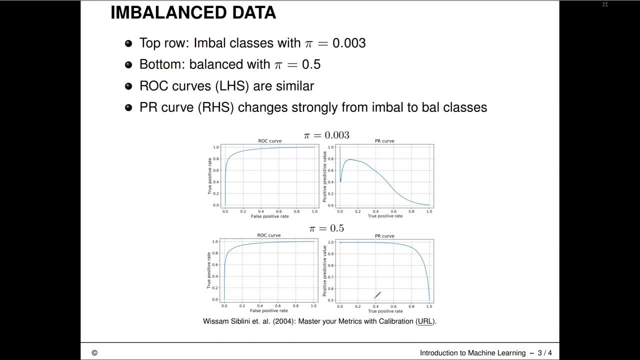 And this is a bit more visible by considering these two guys Instead of this and this guy. again similar analysis. So we see here one classifier evaluated on again a fairly well actually evaluated on two situations. So in the top row we see the situation of imbalance classes and in the bottom we have 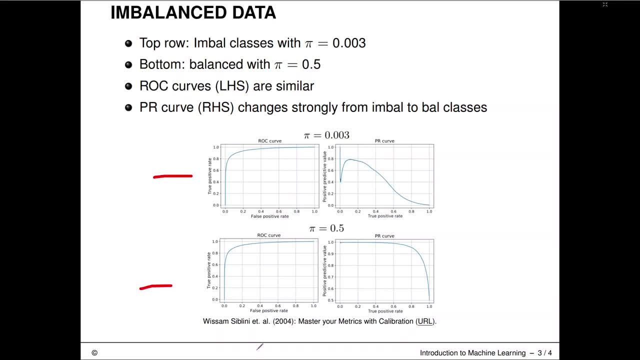 a fairly balanced situation. So it's the same underlying data generating process, the same distribution, the same classifier, But what we are changing is the balance. You have the classes in our test set to draw the curves, So here it's 50: 50.. 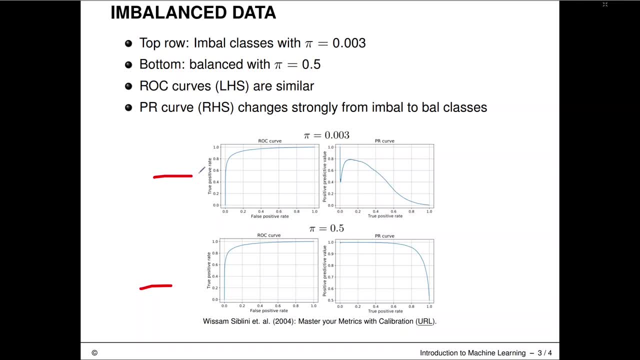 Here it's fairly imbalanced. So here the negative class is much, much larger. If you look at the ROC curves- of the ROC curves you see here in the first, in the first column, you can see that they are. they are both looking quite OK. 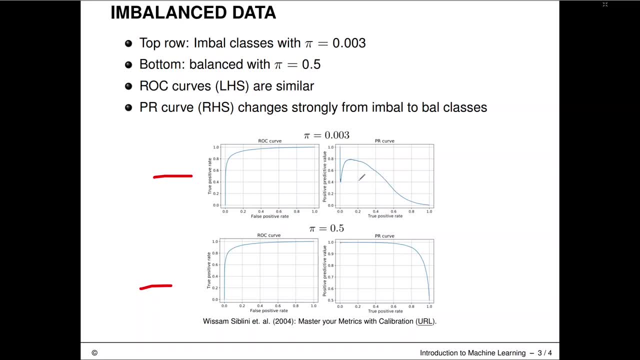 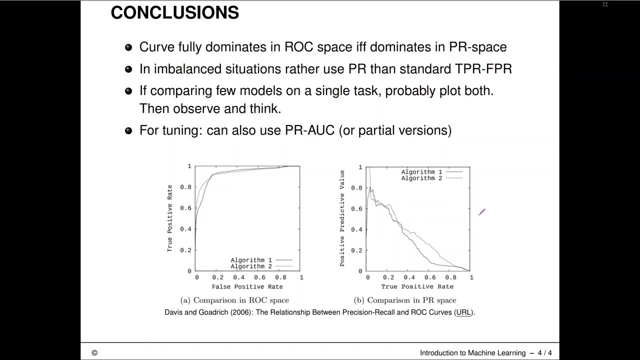 While in the second column you can see that the PR curve actually shows that the classifier does not work very well in the imbalance case here. So conclusions: So so, first of all, what is good to know is that a curve fully dominates another curve in ROC space if, and only if, it dominates in PR space.